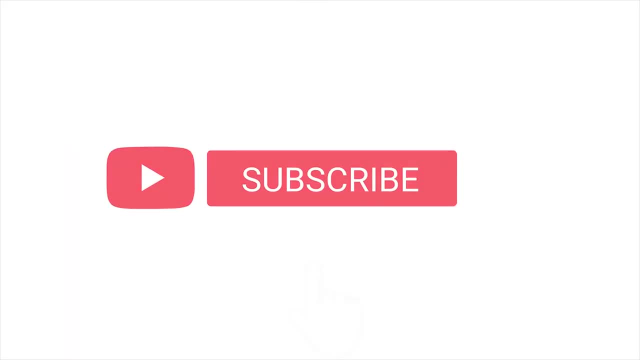 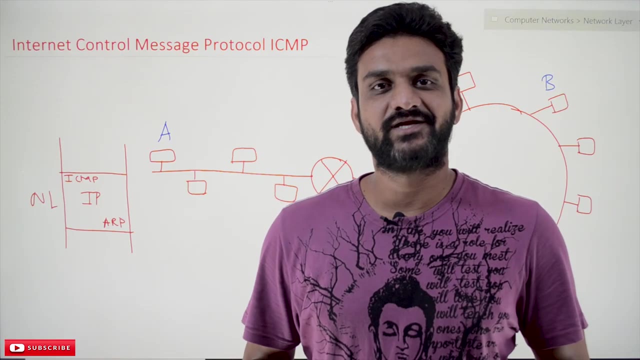 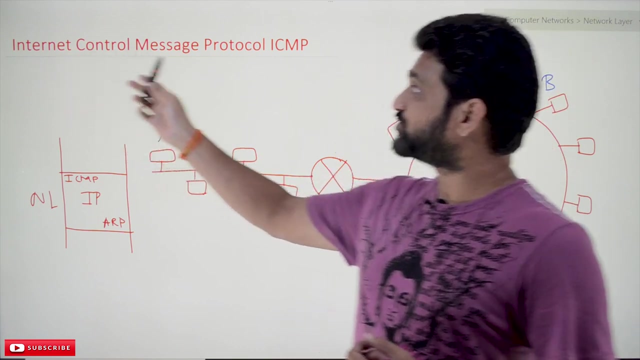 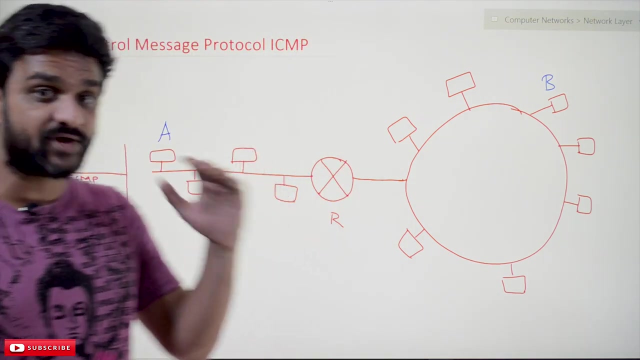 Hi, welcome to Learning Monkey. I am Vikram. In this class we will try to understand ICMP. It is Internet Control Message Protocol, In short it is ICMP. So the ICMP protocol is a network layer protocol. So apart from IPARP we also have another protocol. So in our previous video where we have discussed 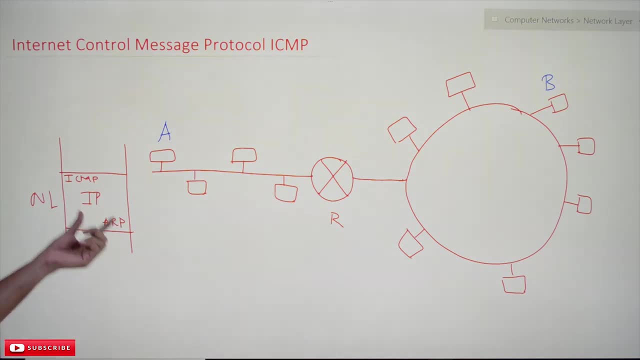 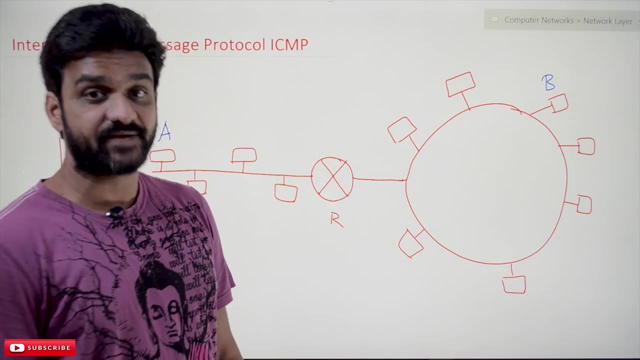 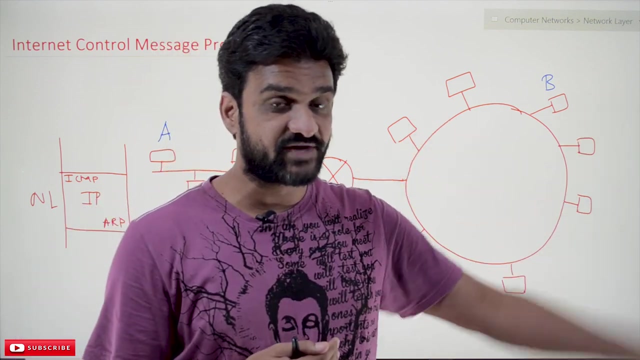 about ARP. we have discussed that. Apart from these, we also have another protocol called ICMP. So what this ICMP will do is it is going to generate error messages, So errors that are generated in the process of transmitting the data from source to destination. 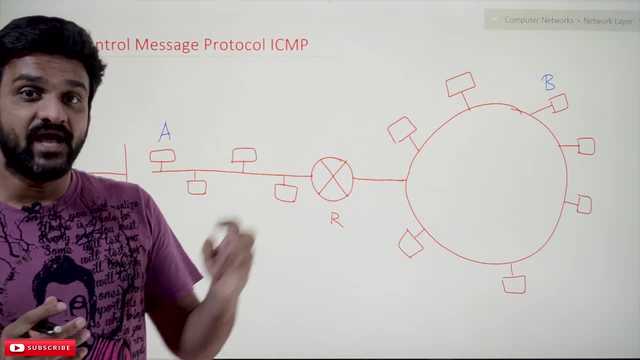 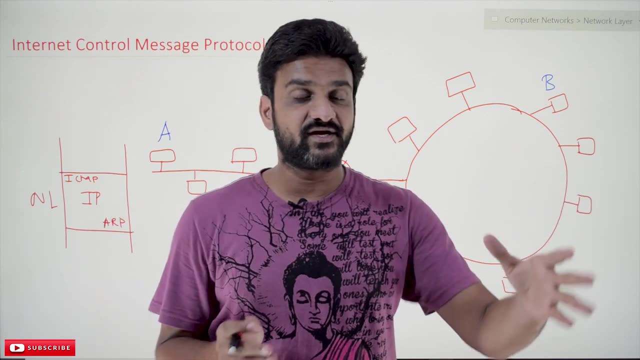 There are different types of error messages that are being generated and they will intimate the source that this kind of error message has been occurred. So in the transmission, if an error occurs, we don't know whether the transmission is done successfully or not. What kind of error has been? 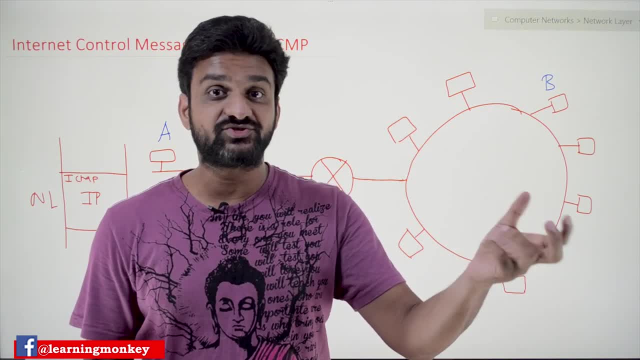 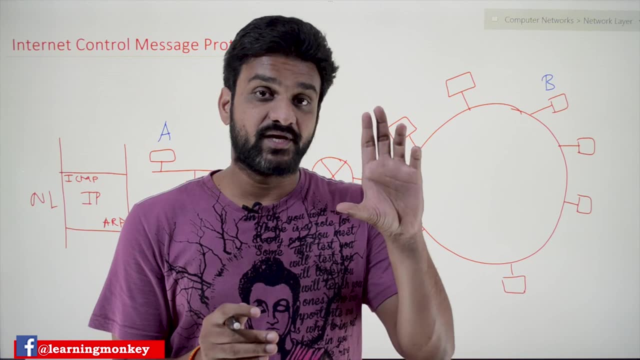 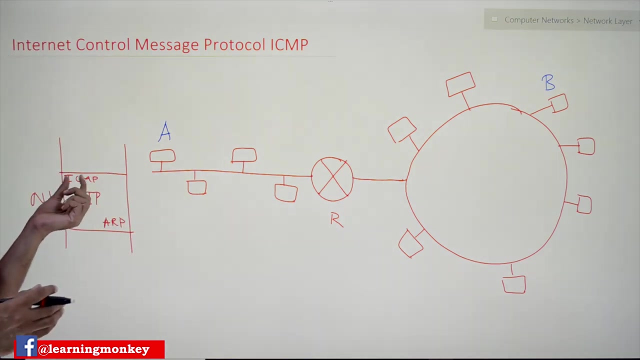 occurred and how that error can be resolved. So the decision has to be taken by the source right. So for that to happen, the network layer is having a process called ICMP. So what this ICMP is? Internet Control Message Protocol. So in that it is going to send the control messages, or error. 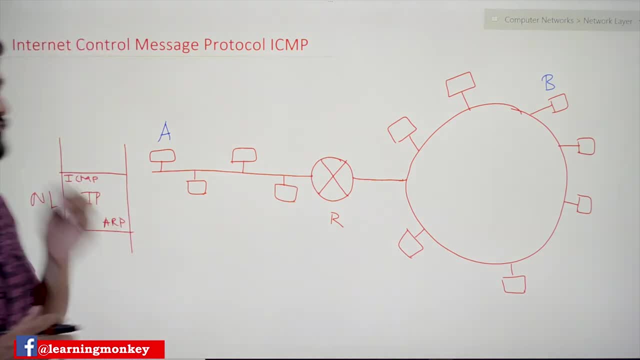 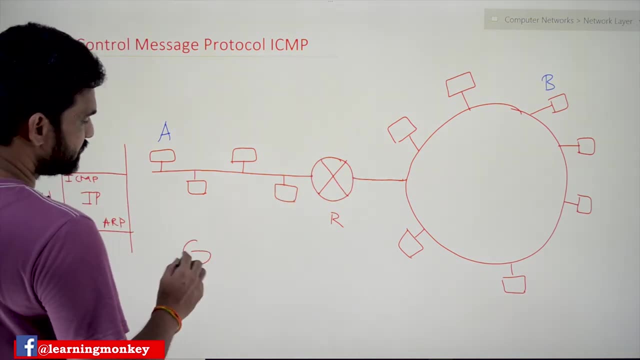 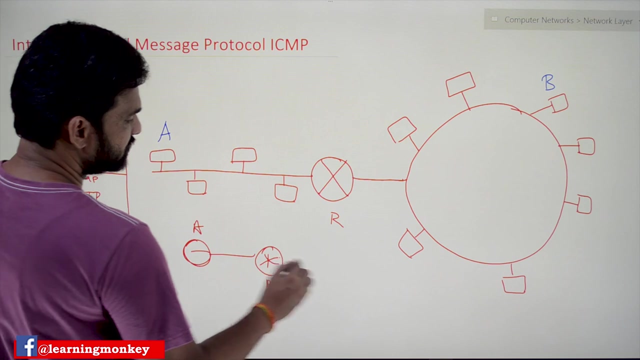 messages to the source. It is going to send the error messages or error messages to the source. So one such kind of error message is Congestion Control Message. For example, if there is a system called A and in this we are having routers, We are having routers in this way and it wants to. 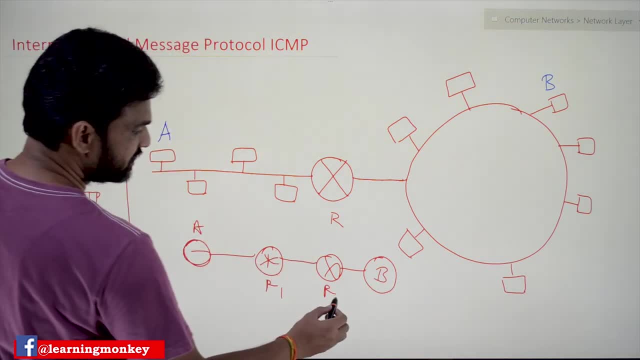 communicate with B. A wants to communicate with B, And here, somewhere in- Assume that it is a router, and this, this system is going to communicate with B, And here, somewhere in- Assume that it is a router, And this, this system is going to28 00. 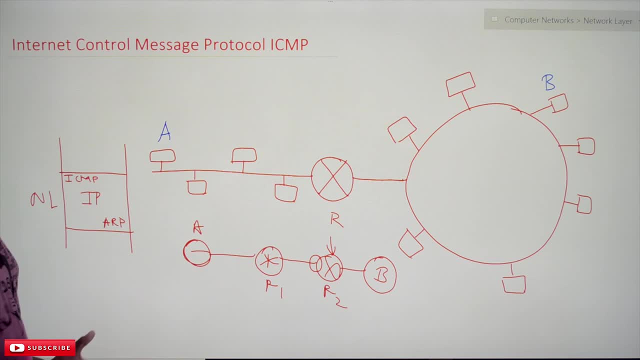 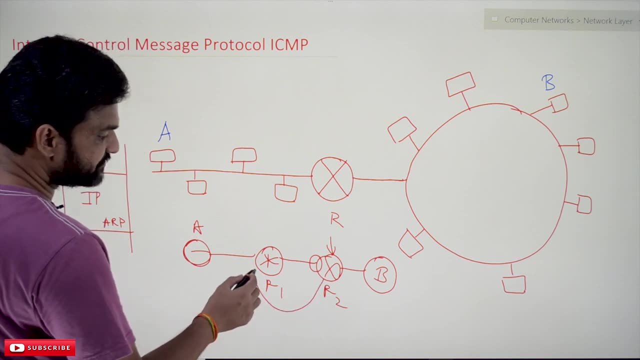 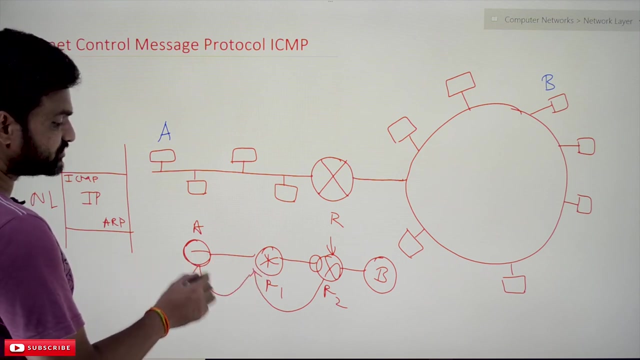 router is congested, so it is having too much of load and it cannot accommodate the packets. so, in that case, so this router will send an icmp packet- icmp packet stating that i am congested with heavy load, so that message will get received at the receiver, at the source, and the source is going. 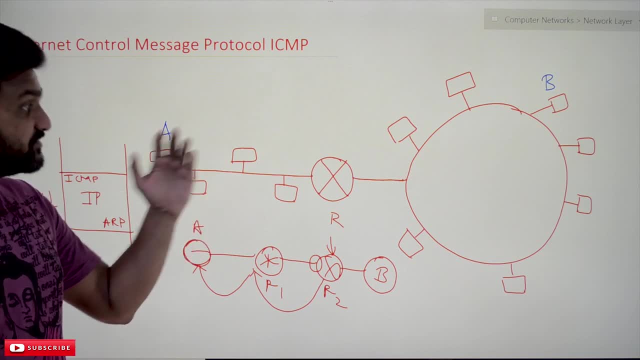 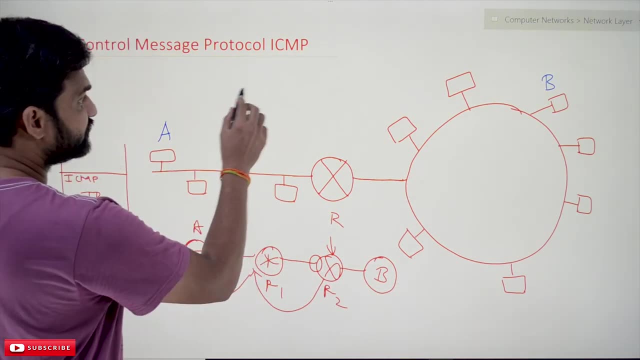 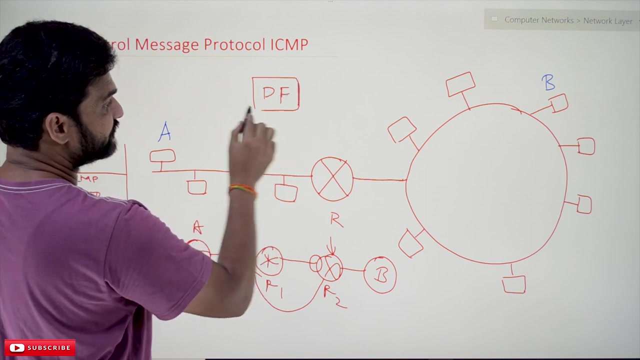 to take the necessary action in that similar way. for example, consider this network. it is don't fragment. so in our network packet we have seen a df, a field cad, in the ipv header we have seen a field called df. in the second row of the ipv header we have seen df. df means do not fragment. 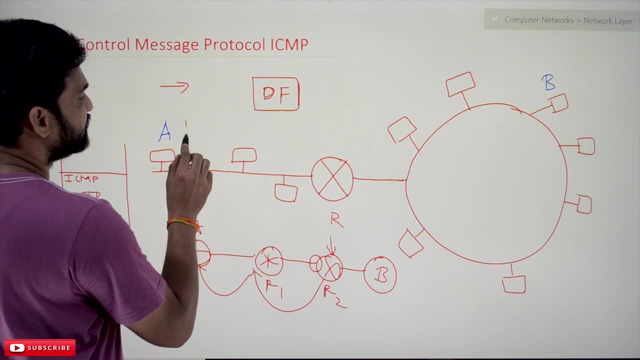 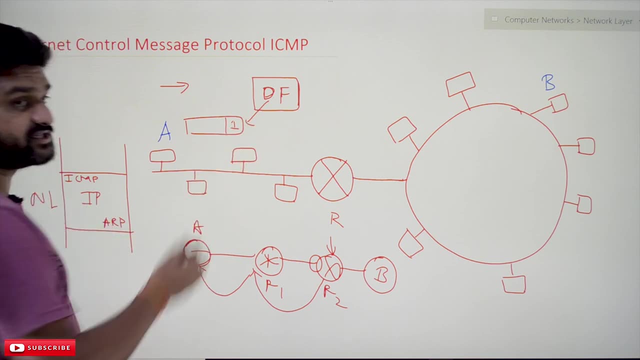 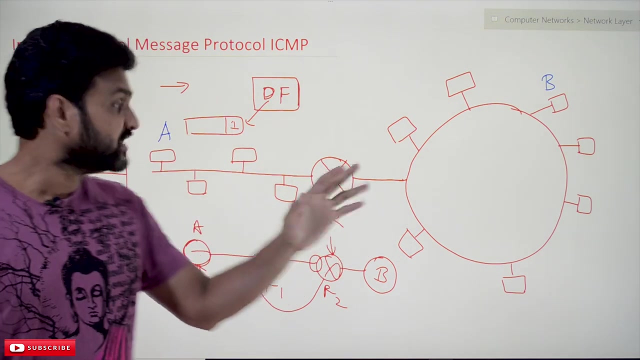 what does that mean is, for example, if a is having a packet and if it is setting the df as one, df as one, in the ipv header, the df is set to one. it means that the packet that is being transmitted- you should not fragment it. for example, if this is, this is having a capacity. 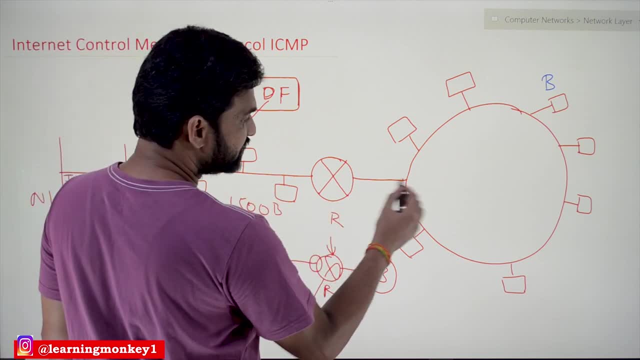 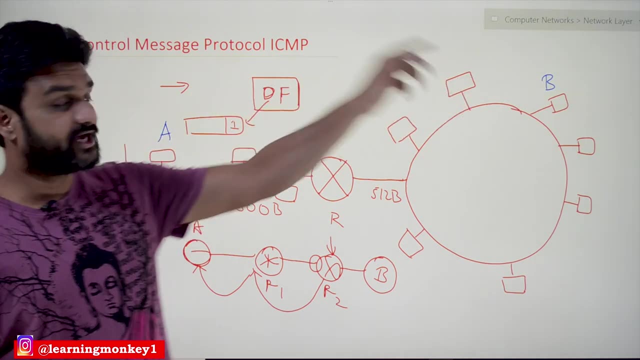 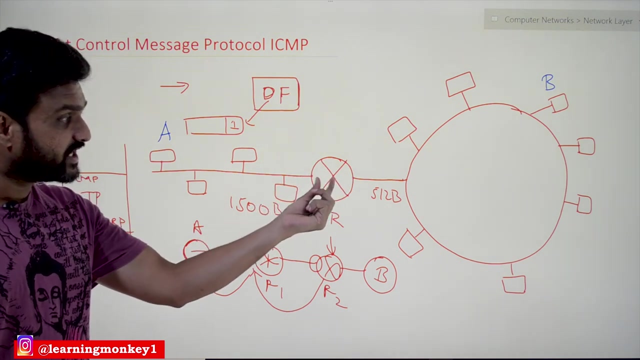 of 1500 bytes. this ethernet and this network is having a capacity of 512 bytes now in order to send the data from a to b, a to b, so 1500 bytes will get transmitted through this network and here at the router. this router has to make the decision that it has to make that 1500 bytes. 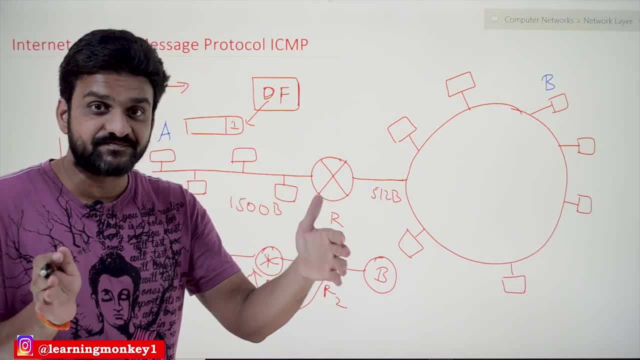 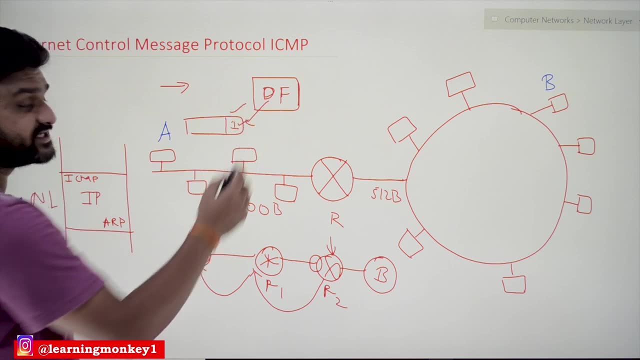 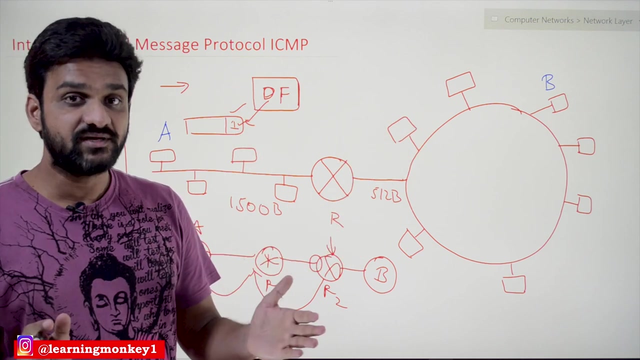 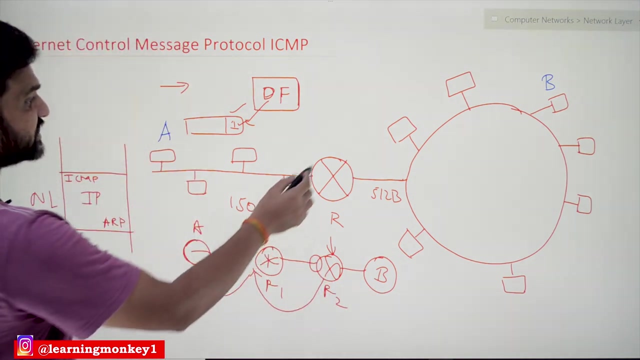 piece of into small, small pieces, into 512 bytes. but what we have set in the IPV header, we have said that don't fragment is set means you don't have the routers in between, you don't have the right to fragment, the right to fragment the packet. so in that, in that case, what the router will do is it will send a ICMP. 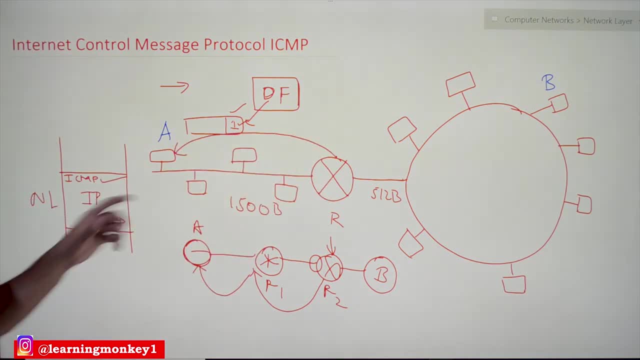 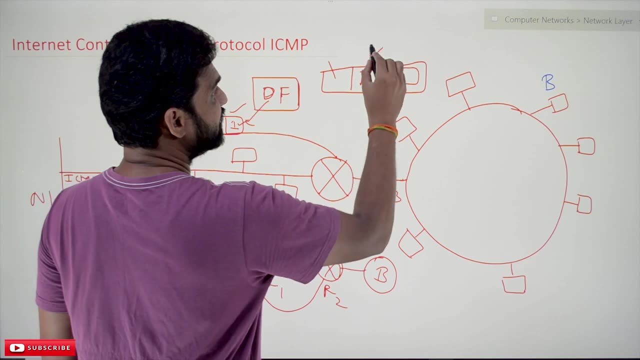 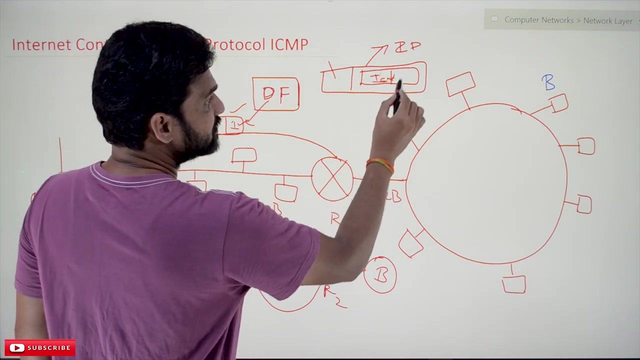 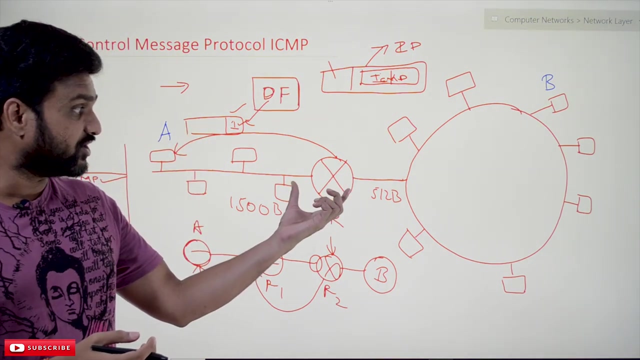 ICMP packet. ICMP packet stating that: and this ICMP is again embedded in the IP, this is the IP header and this is the IP packet. IP packet and within this we are going to send the ICMP packet. this is ICMP packet. so what it states is: you are, you are telling me that I should not fragment, but there is, in order for the. 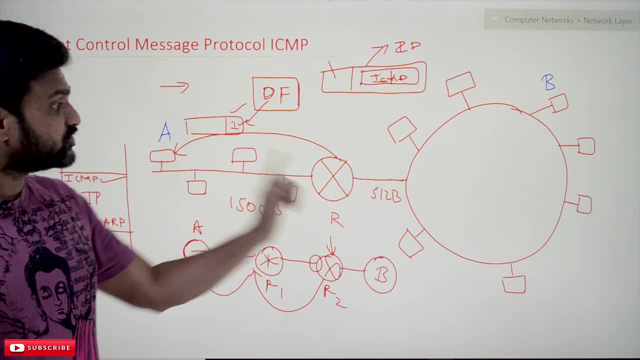 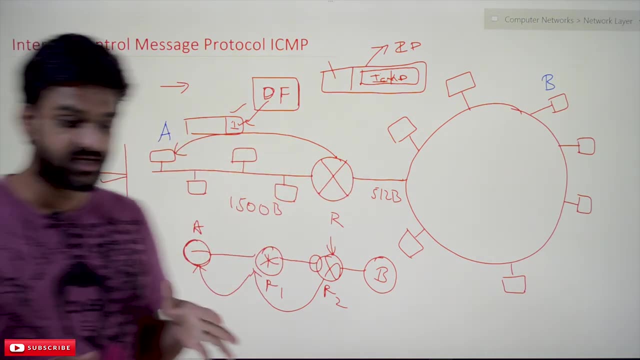 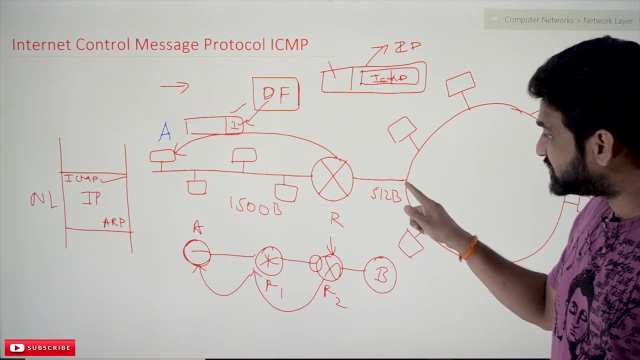 further transmission I want this packet to be transmitting, transmitted to the packet into 512 bytes. so this request will be transmitted. so what the source will do is now, it will make the packet into small, small pieces so that it can accommodate it, so that it can transmit it data. so this 515 hundred bytes of